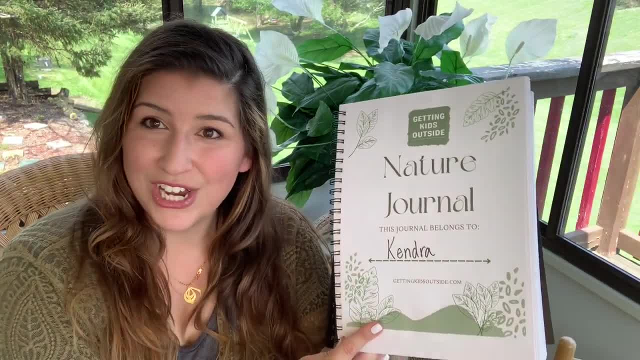 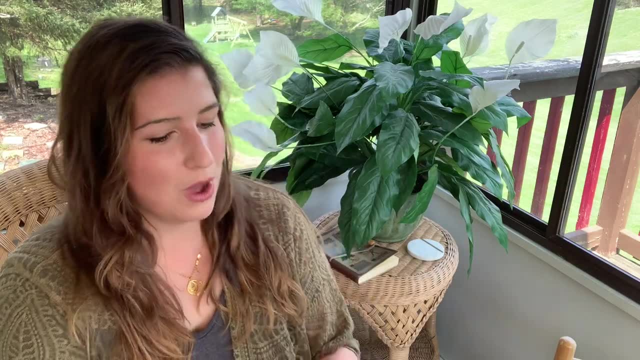 out the pdf and we glued each page in, So I'm going to show you what that looks like. I'll show you a video of me creating mine, and also what it looks like having toddlers create one as well. There are different versions of the pages, So, as you can see, this is an 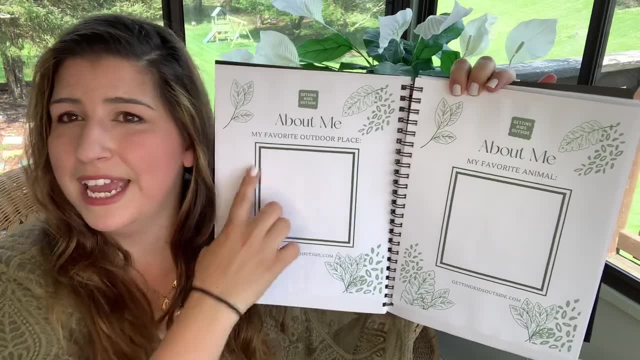 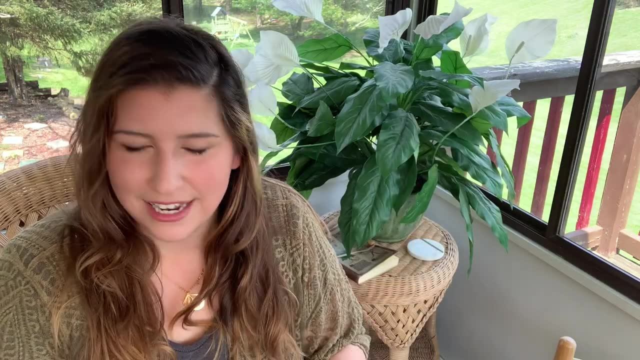 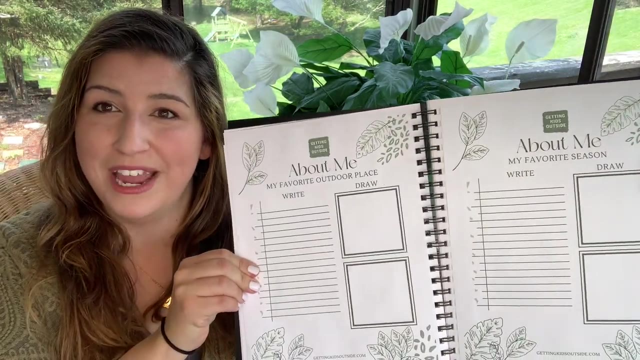 about me page. This one is specifically more for toddlers. It's just a big space for them to draw. It asks: my favorite outdoor place, my favorite animal, my favorite season, things like that. And you will see the exact same questions asked in a different format on some of the other pages. 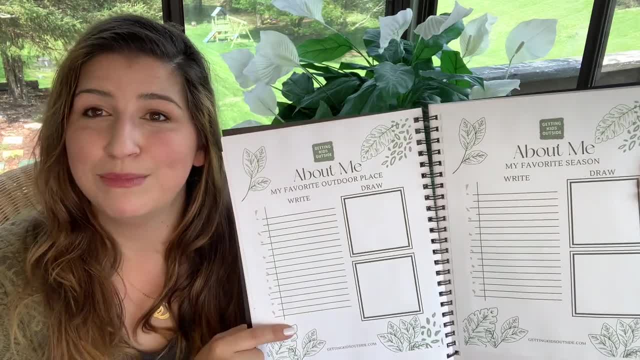 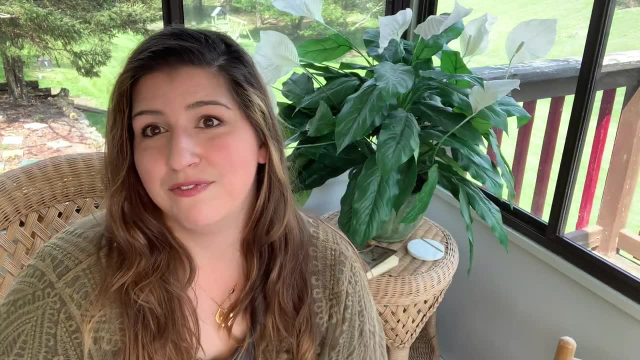 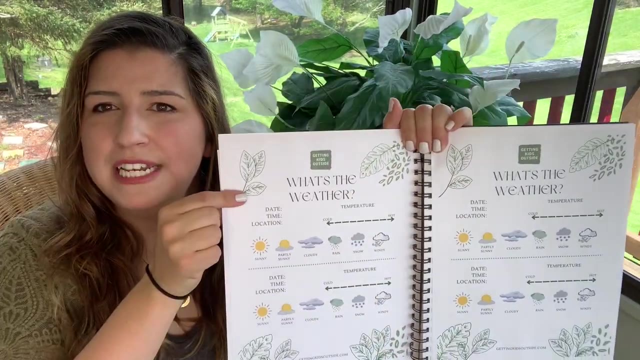 So this is the same exact thing, except you'll notice there's a place for them to write full sentences and to draw. So, depending on the age of your children, you can customize it however fits best for you. Another fun feature that I decided to make is a what's the weather page. Now, each of these: 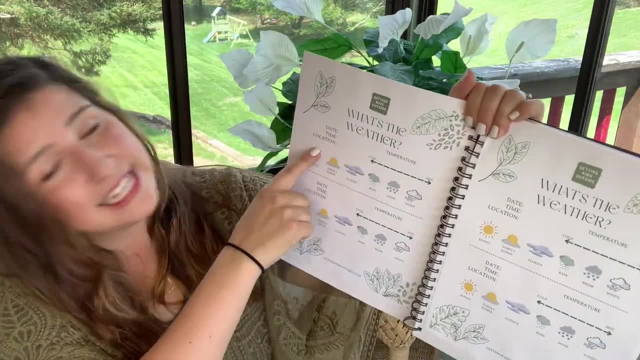 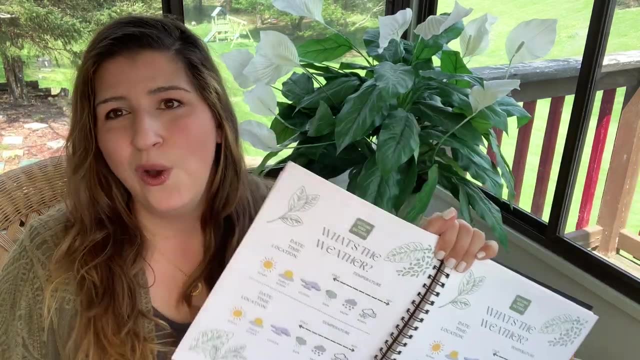 actually half of the page is one day, So you can mark the date, the time, the location, and then you can mark the weather and the temperature Again. you could print out a ton of these and do it every single day, or you could just do it every once in a while. 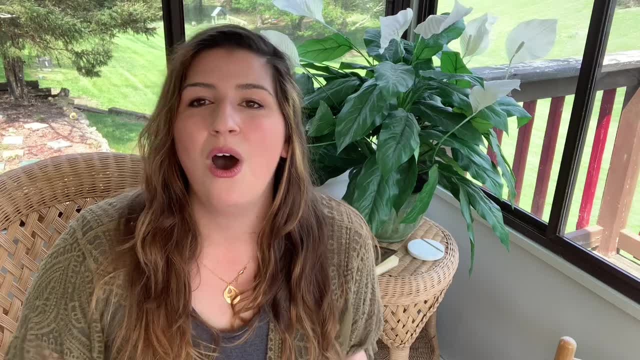 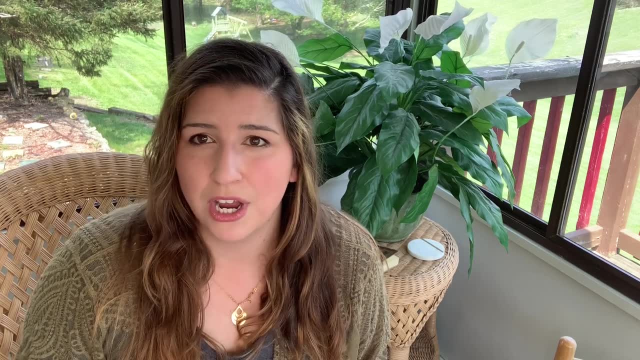 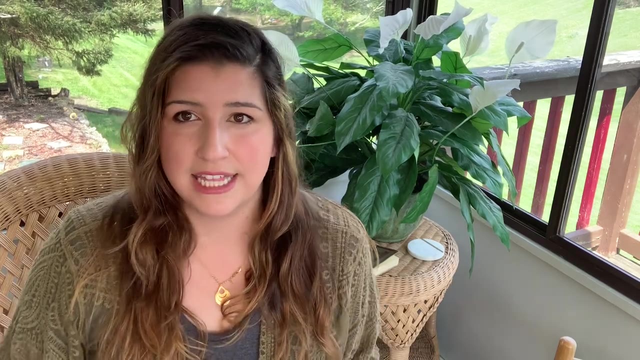 or skip this page altogether. It's totally up to you. All of the activities that I am giving this summer are very easy: Going outside, picking flowers, looking at what animals are in your yard, looking around where you live- Very easy. However, all of them can very easily be taken to the next. 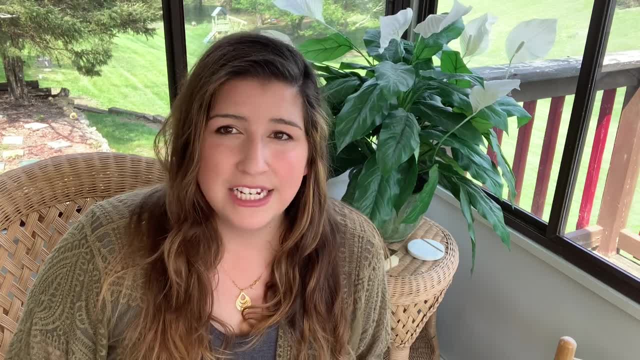 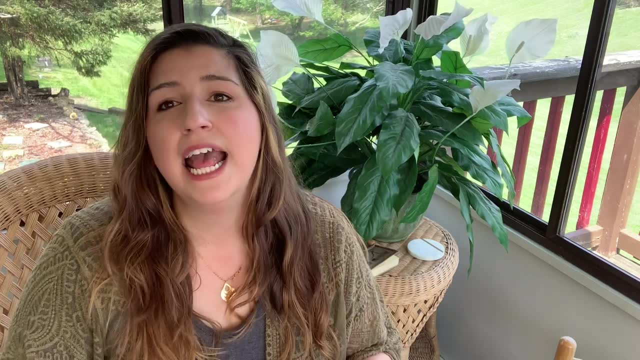 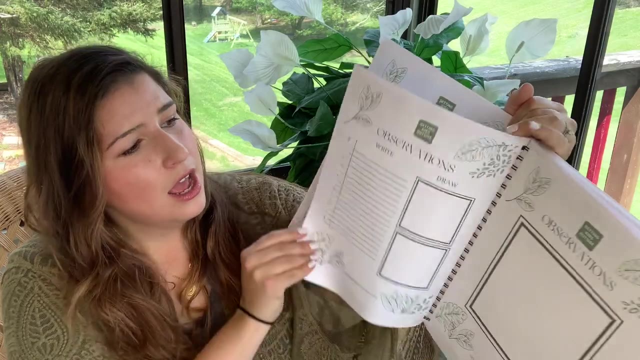 level in terms of educational value. Each of the activities is linked specifically to some sort of STEM-based learning, And so you're going to see that in each of the video I encourage you to take notes and to record observations. So you're going to see those page options in the PDF file. 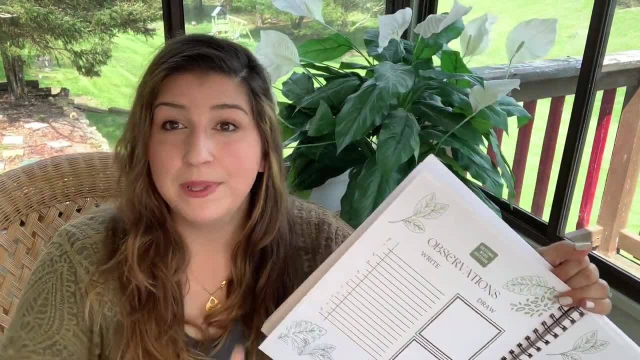 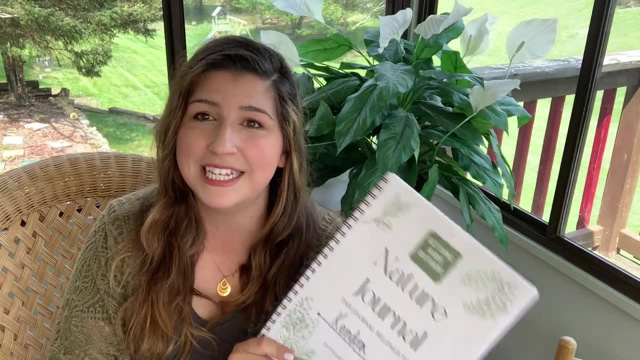 I created just one of each in the PDF, but then you can print as many copies as you need for each of the activities. So now that I've sort of given you a tour of what you will see in the Nature Journal document, take a look at how I put my Nature Journal together and how my boys decided.